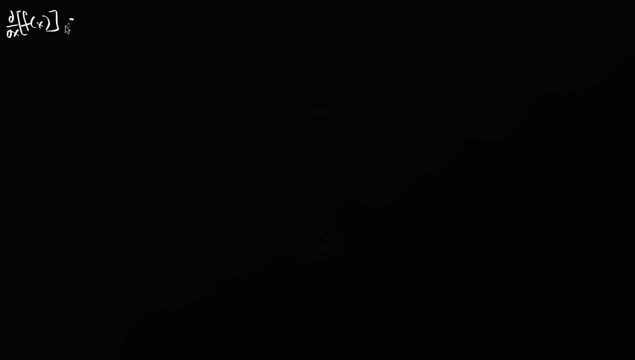 by definition, the derivative of f of x is the limit as h approaches zero, of f of x, plus h, minus f of x, all of that over h. If we want to think of it visually, this is the slope of the tangent line, and all of that. 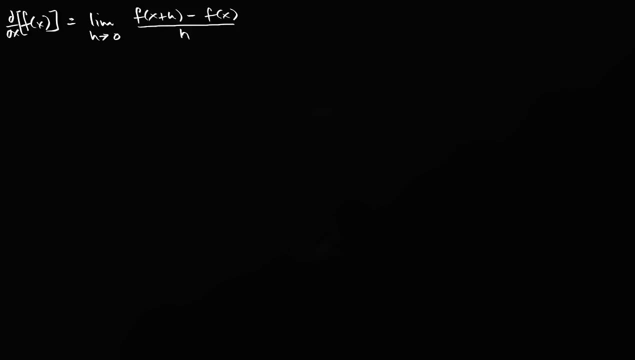 But now I want to do something a little bit more interesting. I want to find the derivative with respect to x, not just of f of x, but the product of two functions: f of x times g of x. And if I can come up with a simple, 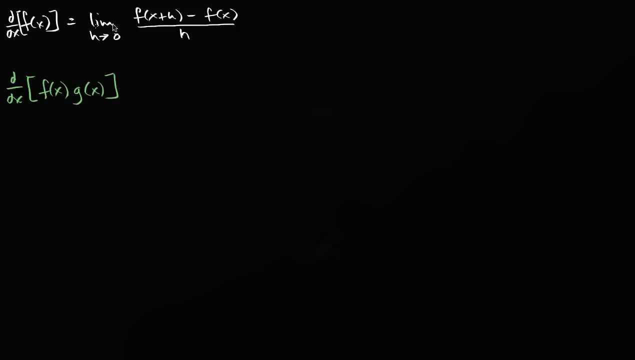 A simple thing for this. that, essentially, is the product rule. Well, if we just apply the definition of a derivative, that means I'm going to take the limit. as h approaches zero In the denominator, I'm going to have an h. 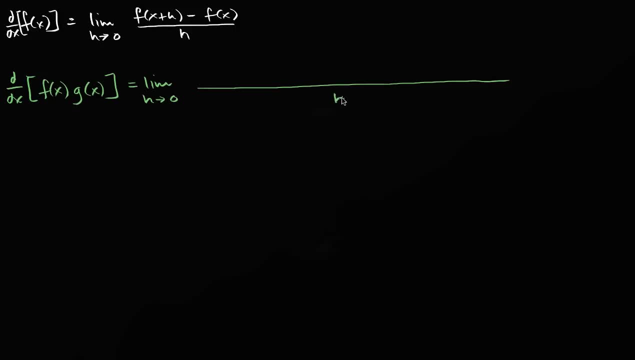 In the denominator I'm going to write a big. It's going to be a big rational expression. In the denominator I'm going to have an h And then I'm going to evaluate this thing at x plus h. So that's going to be f of x plus h, g of x plus h. 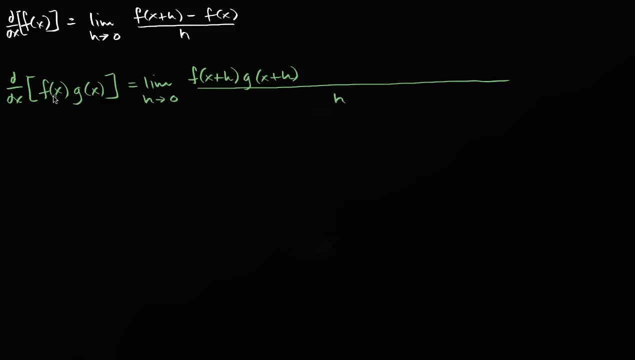 And from that I'm going to subtract this thing evaluated at f of x Or, sorry, this thing evaluated at x. So that's going to be f of x times g of x, And I'm going to put a big awkward space here. 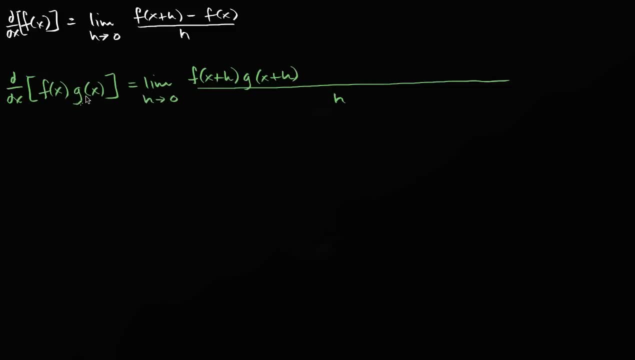 and you're going to see why in a second. So if I evaluate this at x, then it's just going to be minus f of x, g of x. All I did so far is I just applied the definition of the derivative Instead of applying it to f of x. 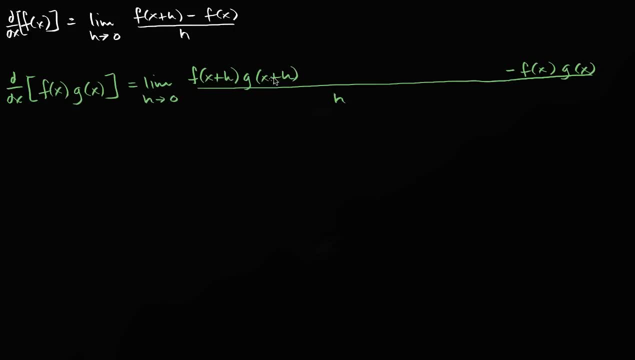 I applied it to f of x times g of x. So you have f of x plus h, g of x plus h, minus f of x, g of x. all of that over h Limit as h approaches zero. Now why did I put this big awkward space here? 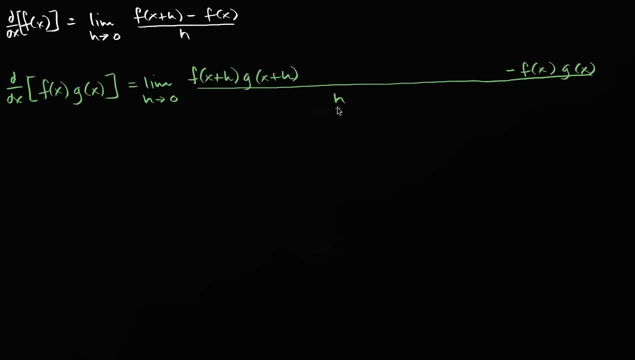 Because, just the way I've written it, right now it doesn't seem easy to algebraically manipulate. I don't know how to evaluate this limit. There doesn't seem to be anything obvious to do, And what I'm about to show you. 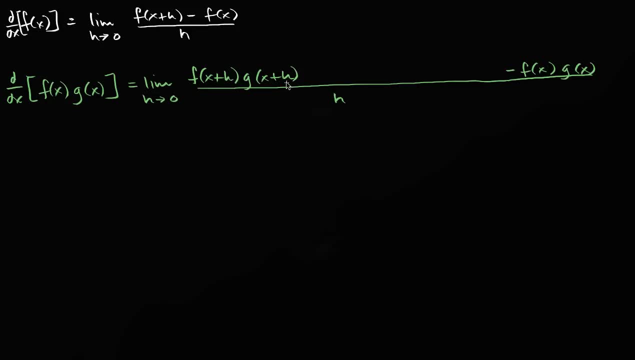 I guess you could view it as a little bit of a trick. I can't claim that I would have figured it out on my own. maybe eventually, if I were spending hours on it, And I'm assuming somebody was fumbling with it long enough. 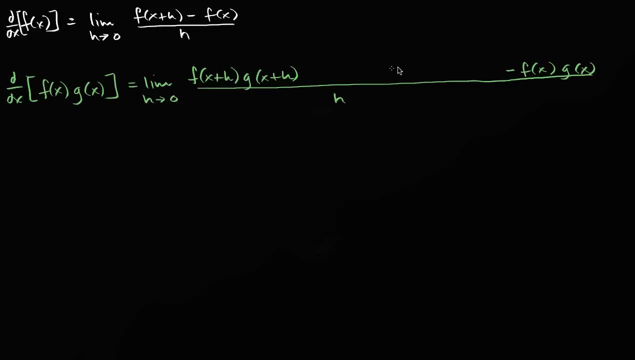 They said: oh wait, wait. Look, if I just add and subtract the same term here, I can begin to algebraically manipulate it and get it to what we all know is the classic product rule. So what do I add and subtract here? 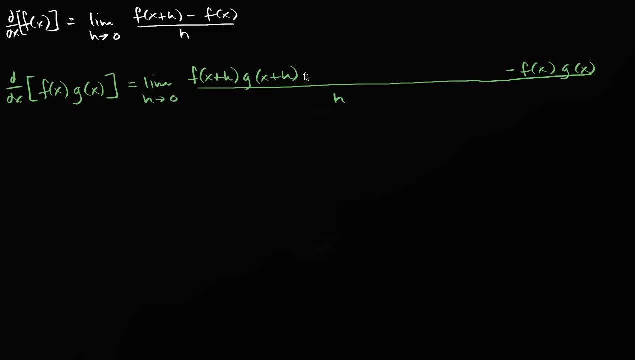 Well, let me give you a clue. So if we have plus, actually let me change this: minus f of x, plus h g of x, I can't just subtract it. If I subtract it, I can't subtract it. 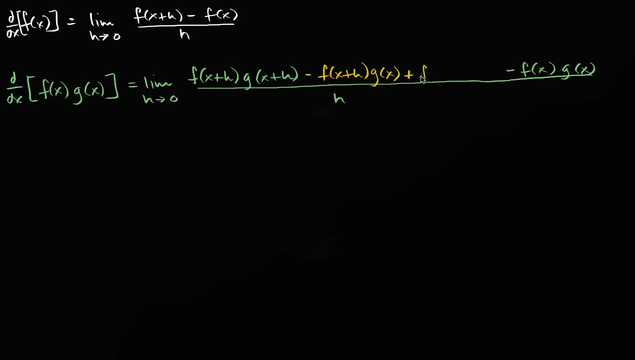 I've got to add it too, so I don't change the value of this expression. So plus f of x, plus h g of x. Now I haven't changed the value, I just added and subtracted the same thing. But now this thing can be manipulated. 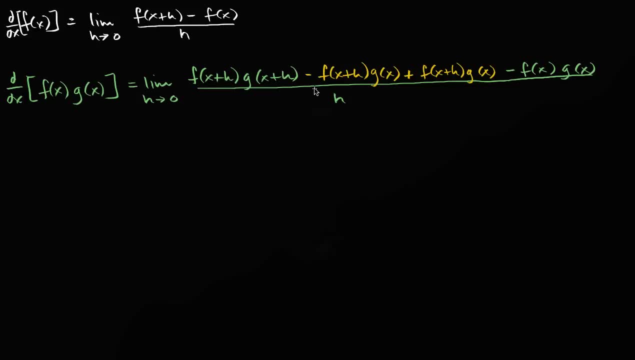 in interesting algebraic ways to get us to what we all love about the product rule. And at any point you get inspired, I encourage you to pause this video. Well, to keep going, let's just keep exploring this expression. So all of this is going to be equal to. 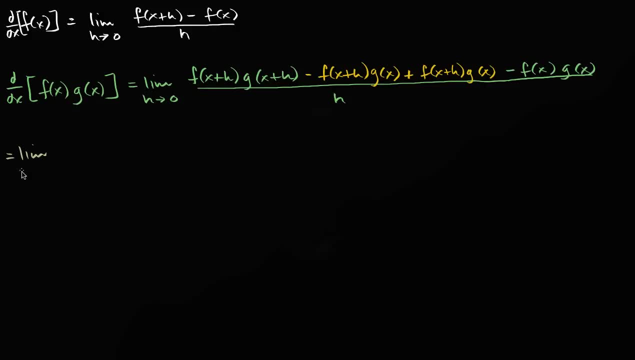 it's all going to be equal to the limit as h approaches zero. So the first thing I'm going to do is I'm going to look at. I'm going to look at this part, this part of the expression And, in particular, let's see. 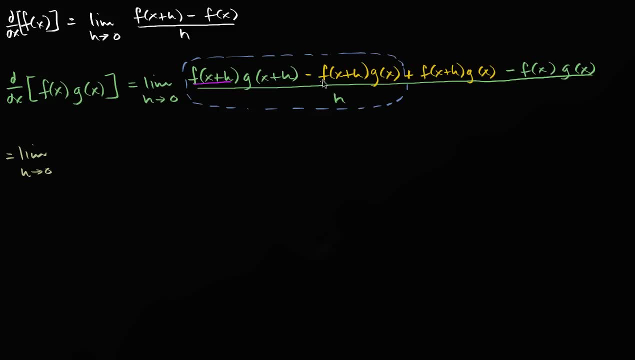 I am going to factor out an f of x plus h. So if you factor out an f of x plus h, this part right over here is going to be f of x plus h. f of x plus h times. you're going to be left with g of x plus h. 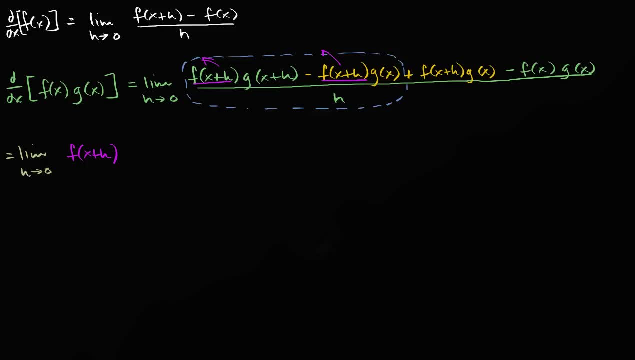 g of. it's a slightly shader, different shade of green g of x plus h. that's that there, minus g of x, minus g of x. whoops, I forgot the parentheses. Oh, it's a different color. 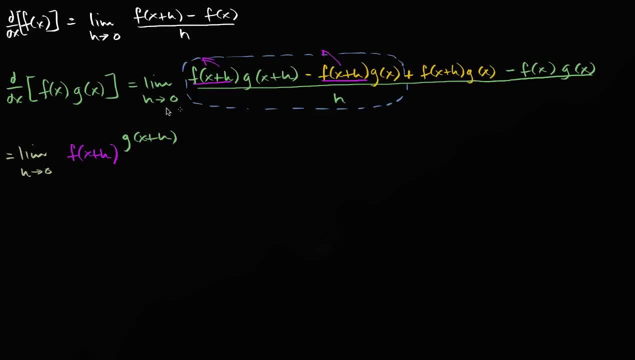 I got a new software program and it's making it hard. It's hard for me to change colors. My apologies, This is not a straightforward proof and the least I could do is change colors more smoothly. All right, g of x plus h minus g of x. 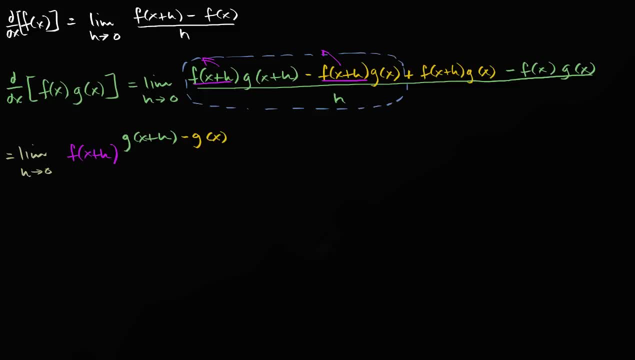 that's that one right over there, and then all of that over this h, all of that over h. so that's this part here, and then this part over here, this part over here, and actually it's still over h. so let me actually 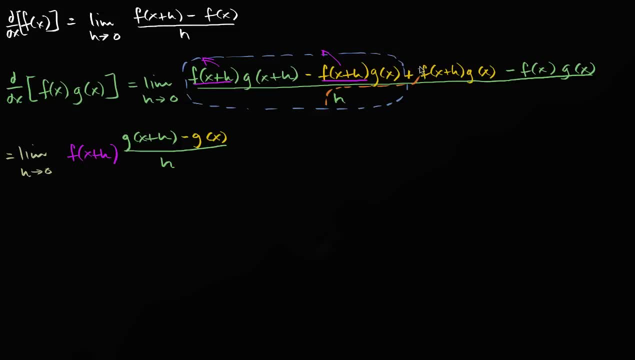 let me circle it like this: So this part over here I can write as: so then we're going to have plus actually here let me factor out a g of x here, So plus g of x, plus g of x times this f of x plus h. 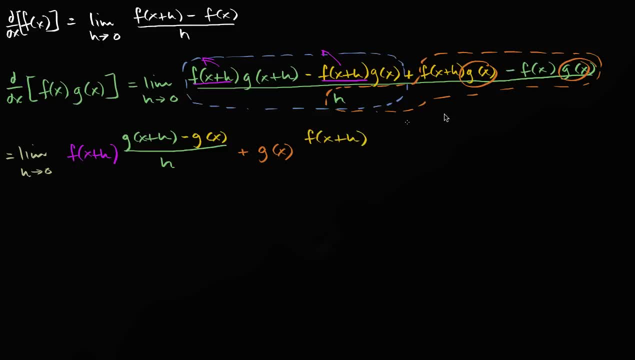 times f of x plus h minus this f of x minus that f of x. all of that over h, all of that over h. Now we know from our limit properties the limit of all of this business. well, that's just going to be the same thing. 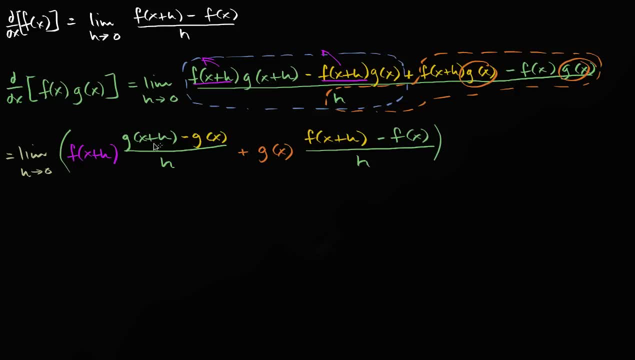 as the limit of this as h approaches zero, plus the limit of this as h approaches zero, and then the limit of the product is going to be the same thing as the product of the limits. So if I use both of those, those limit properties. 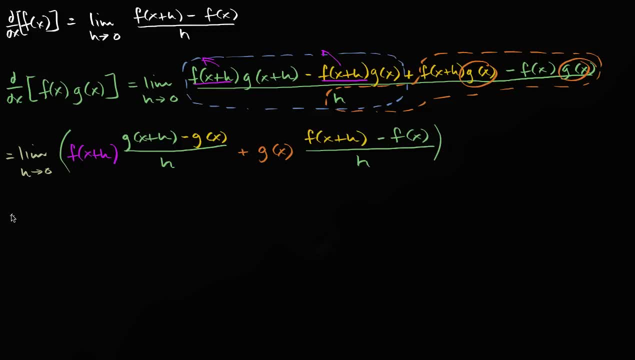 I can rewrite this whole thing as the limit. let me give myself some real estate. the limit as h approaches zero, of f of x plus h, of f of x plus h, times times the limit as h approaches zero of all of this business. 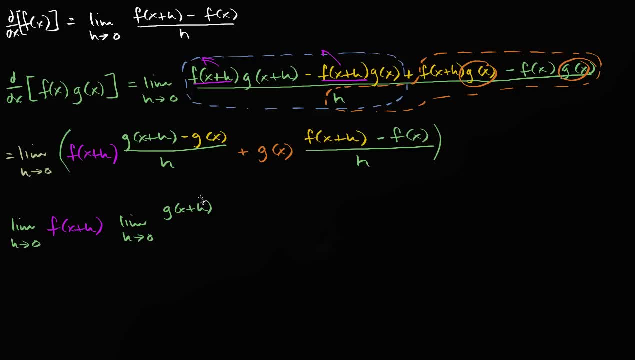 g of x plus h, minus g of x, minus g of x. all of that over h. I think you might see where this is going. very exciting. plus plus the limit. let me write that a little bit more clearly. 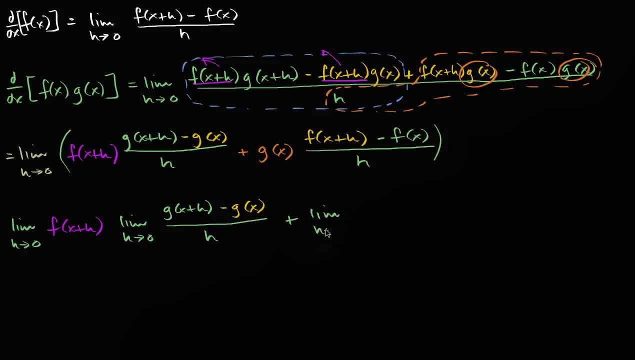 plus the limit as h approaches zero of g of x, our nice brown colored g of x times. now we have a product here. the limit, the limit as h approaches zero of f of x plus h of f of x plus h. 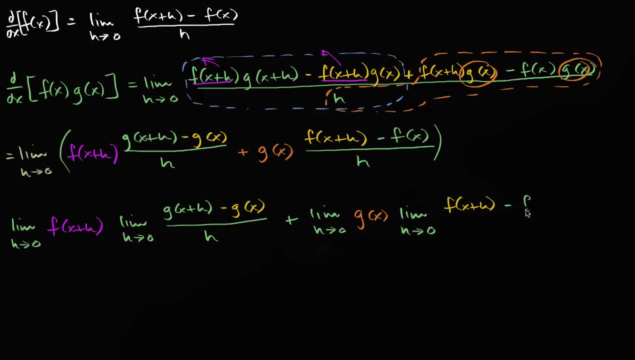 minus f of x, minus f of x, all of that, all of that over h, and let me put the parentheses where they're appropriate so that that that, that And all I did here, the limit, the limit of this sum. 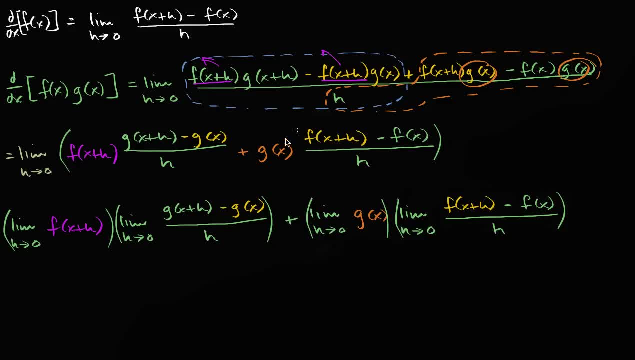 that's going to be the sum of the limits. that's going to be the limit of this plus the limit of that, and then the limit of the products is going to be the same thing as the product of the limits. so I just used those limit properties here. 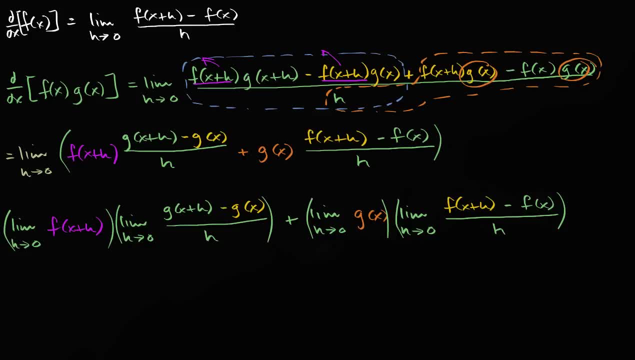 but now let's evaluate them. what's the limit? and I'll do it in different colors. what's this thing right over here? the limit, as h approaches zero of f of x plus h. well, that's just going to be f of x. 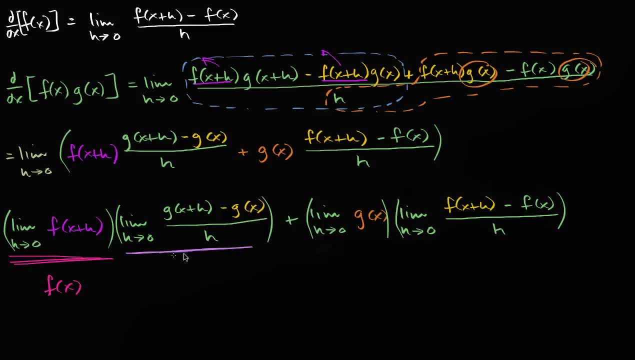 now, this is the exciting part. what is this? the limit, as h approaches zero, of g of x plus h, minus g of x over h. well, that's just our, that's the definition of our derivative, that's the derivative of g. 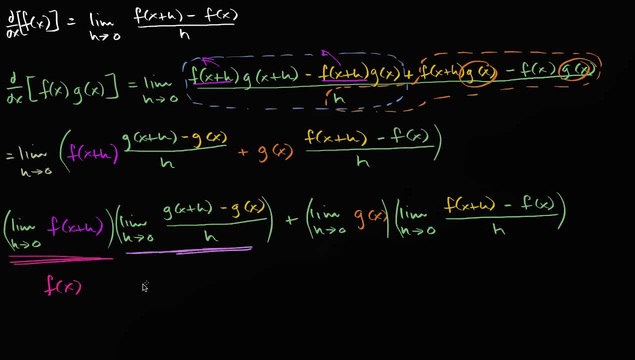 so this is going to be, this is going to be the derivative of g of x, which is going to be g prime of x, g prime of x. so you're multiplying these two and then you're going to have plus- what's the limit as h approaches zero of g of x. 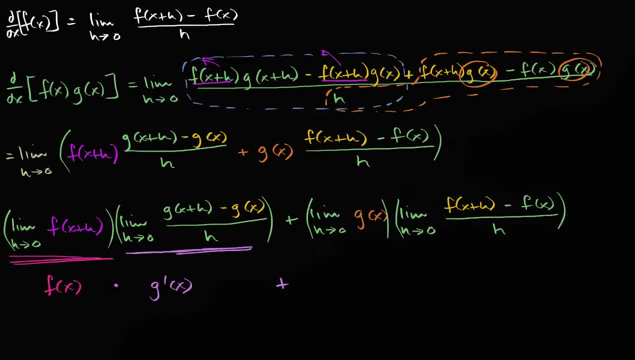 well, there's not even any h in here, so this is just going to be g of x, so plus g of x times the limit. so let's see, this one is in brown and the last one I'll do in yellow. 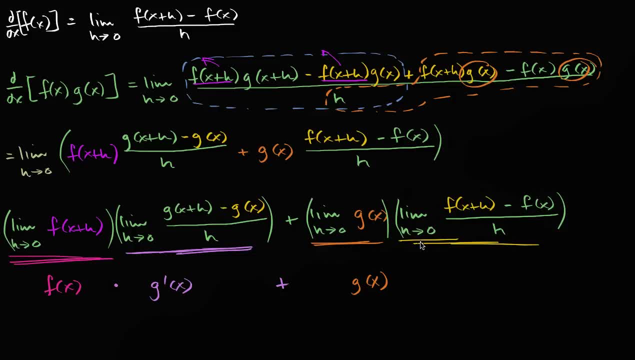 times the limit as h approaches zero. and we're getting very close. the drum roll should be starting. limit as h approaches zero of f of x plus h minus. f of x over h. well, that's the definition of the derivative of f of x. 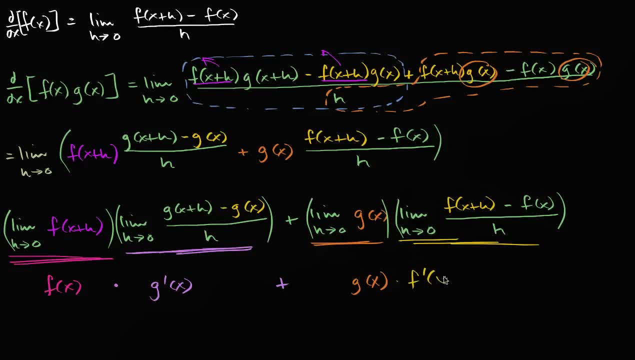 this is f prime of x times f prime of x. so there you have it. the derivative of f of x times g of x is this, and if I wanted to write it in a little bit more condensed form, it is equal to: 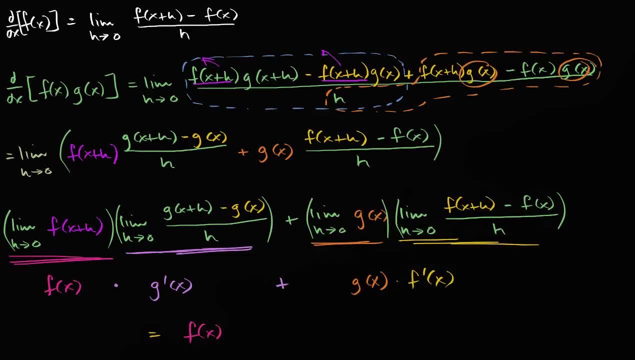 it is equal to f of x times the derivative of g with respect to x times the derivative of g with respect to x plus g of x plus g of x times the derivative of f with respect to x, f with respect to x.